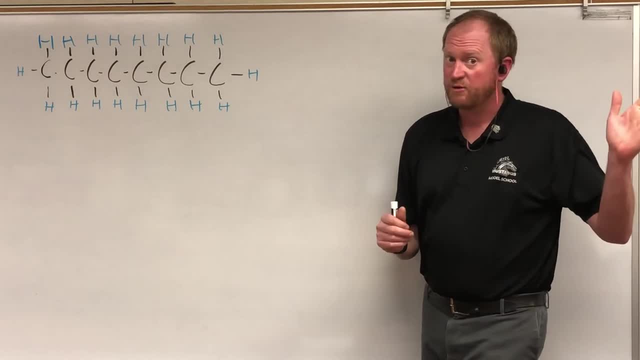 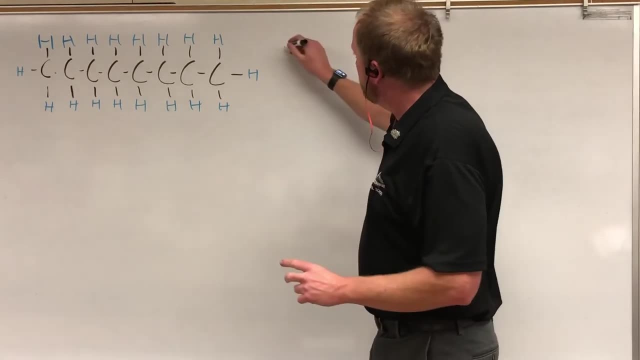 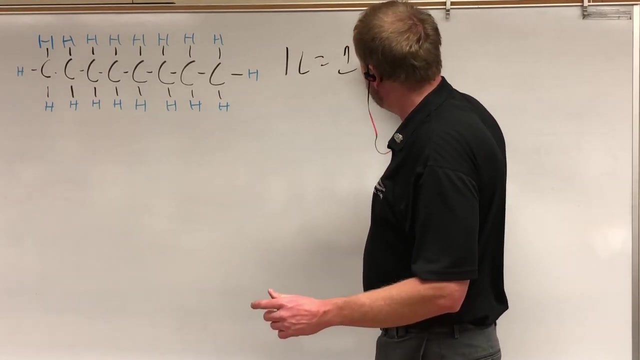 information about what's going into your tank and figure out how much carbon dioxide is going out the tail, And I'll show you how. Let's start with the very basics, okay. So, first off, you probably already know that one liter of water is equal to one ton of CO2.. 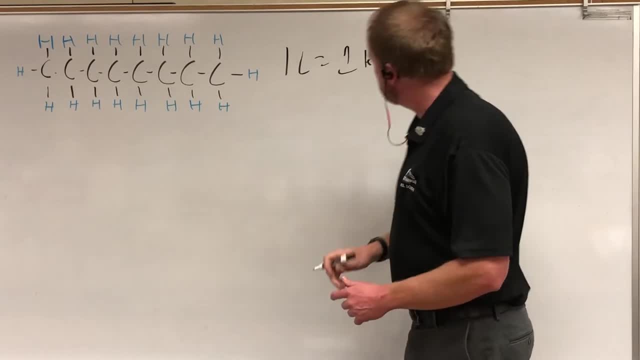 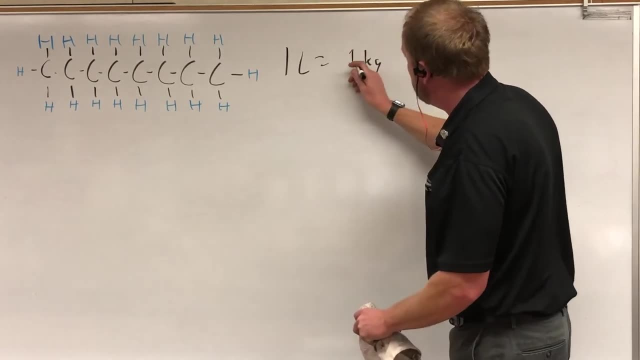 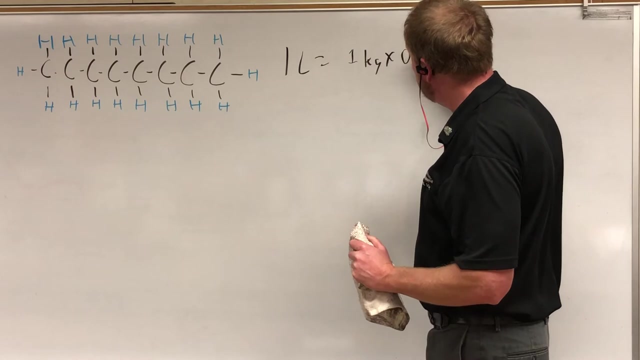 One kilogram, right, And you're off to the races. That's a horrible looking one, isn't it? Let's go with it, though. So you have one kilogram per liter, but that's water. Now, gasoline has a density of 0.703.. Gasoline is less dense than water, That's. 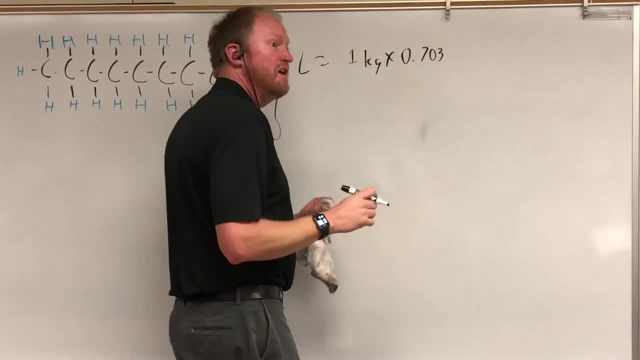 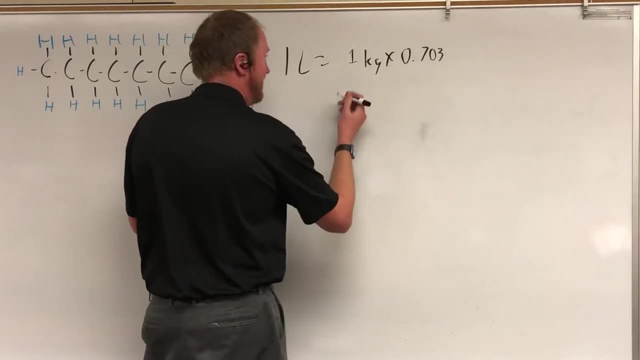 why they tell you not to try to put out a gasoline fire with water, because the water will all end up under the gasoline that still will be burning. But that's not true, Neither here nor there. So you multiply that together and you find that one. 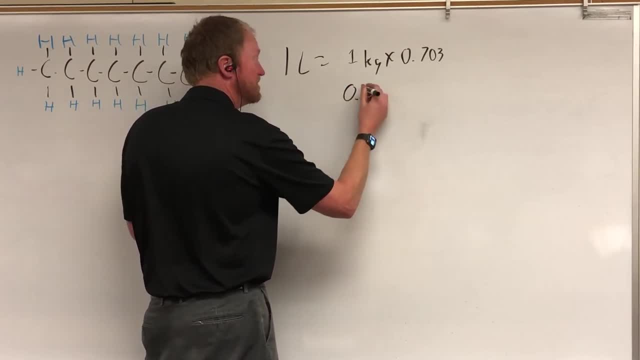 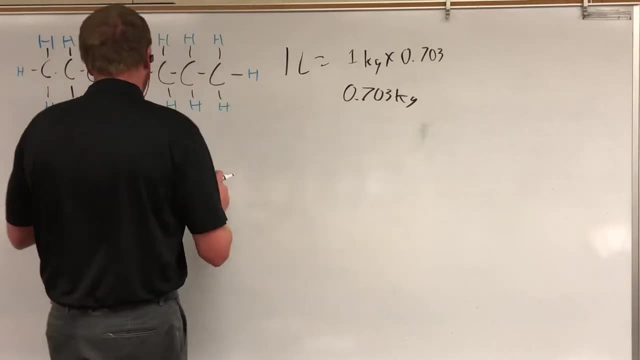 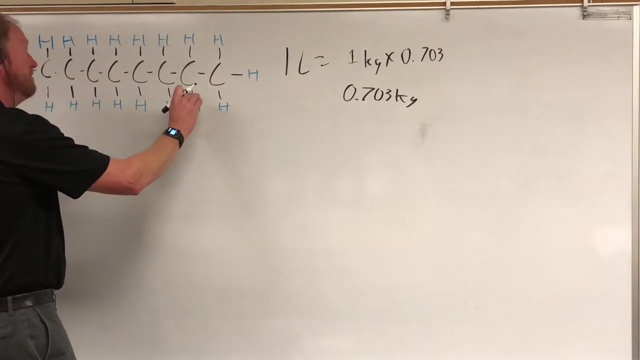 liter of gasoline has a mass of 0.703 kilograms. Now, is that the amount of carbon you're putting up in the air? No, Because gasoline, speaking of gasoline, gasoline is not all carbon. There's carbon: eight atoms of carbon and 18. 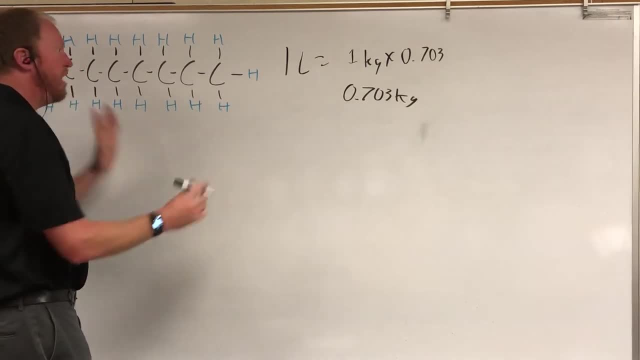 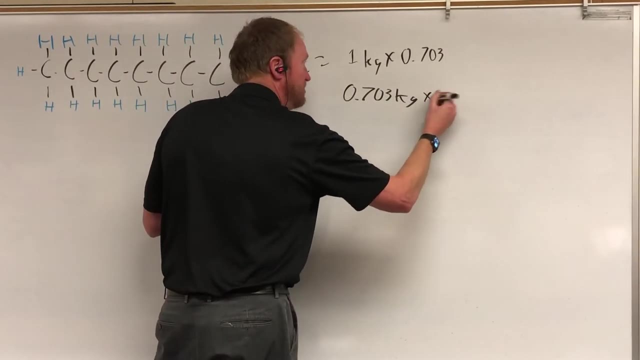 atoms of hydrogen. So we got to actually figure out how much of that- 0.703 kilograms, is the actual carbon. So the way you do that is you basically take the carbon One, two, three, four, five, six, seven, eight. They have eight of them Each. carbon has a molar weight of 12.. So 8 times 12 is 96 out of. well, what is the total? Well, that's 96 plus 18 hydrogen. Each hydrogen is much lighter than carbon- only a molar weight of one. So the total molar weight of the entire molecule. 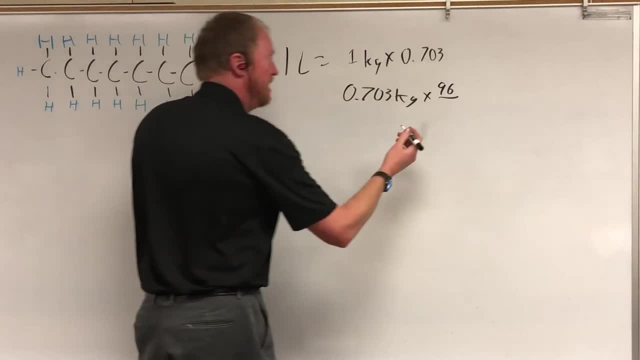 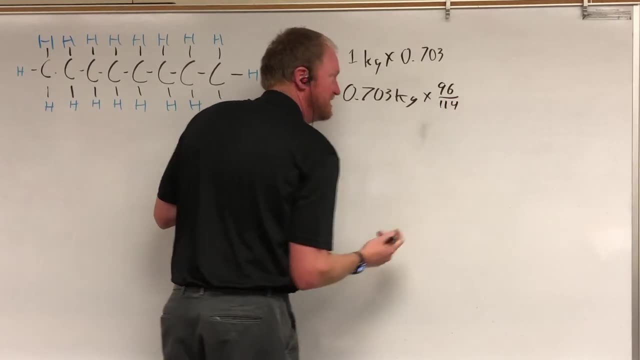 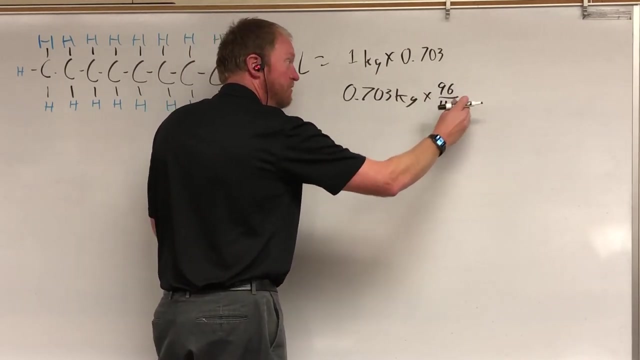 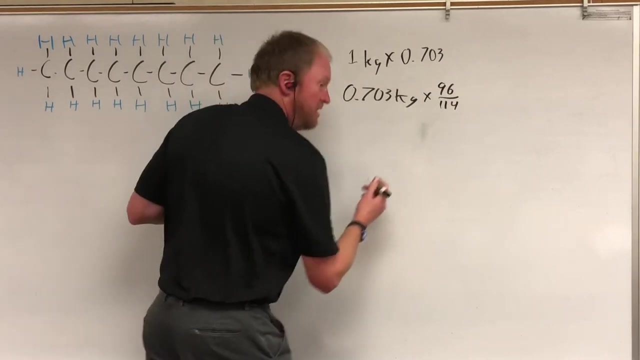 in addition is 96 plus 18, which gives you- oh boy, my mind is stopped, I wrote it down, fortunately- 114.. So 96 grams out of 114 grams for one mole of gasoline is carbon. So multiply that together and you find that of that 0.73 kilograms, you end. 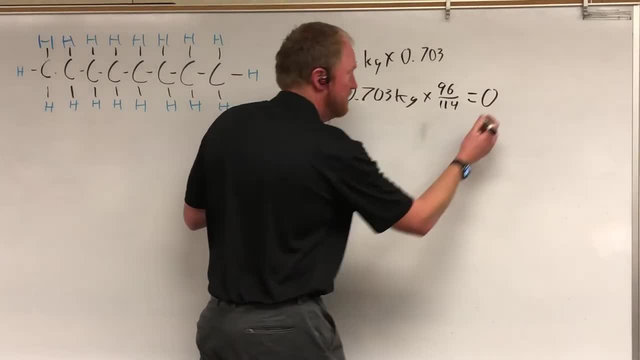 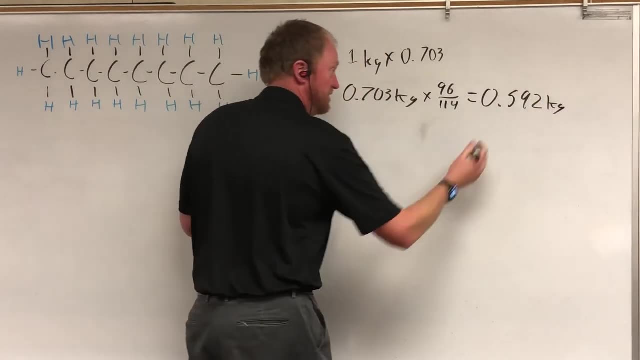 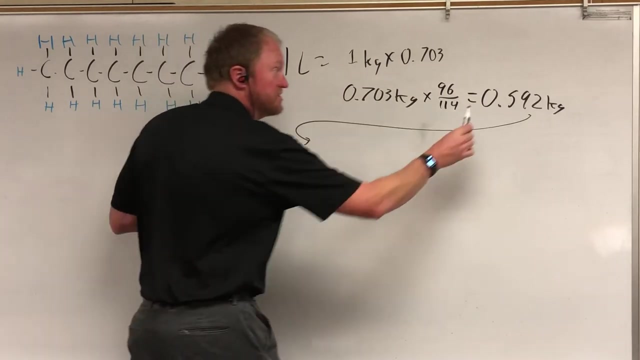 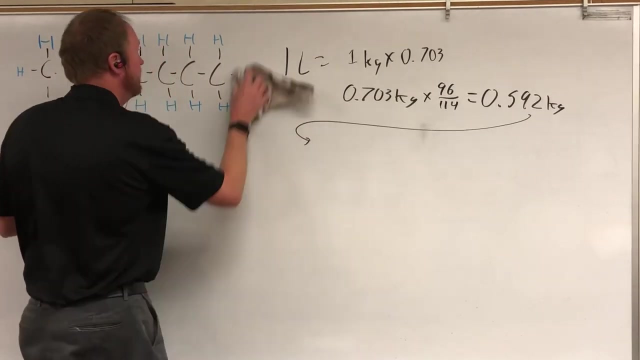 up with zero point five nine two kilograms of carbon in your liter of gasoline. now let's take that a little further. so if you burn that, you don't get zero point five nine two kilograms of carbon dioxide. here's the reason why every carbon, when you break it away from the gasoline, combines with two atoms of. 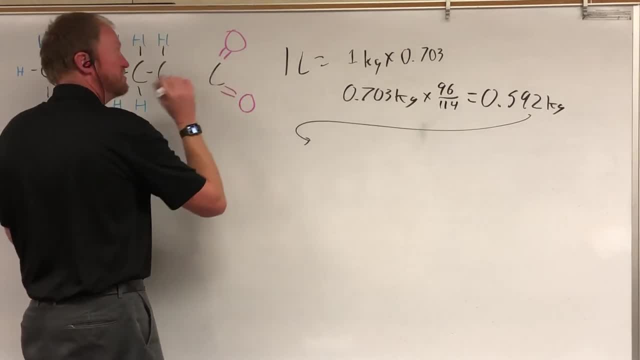 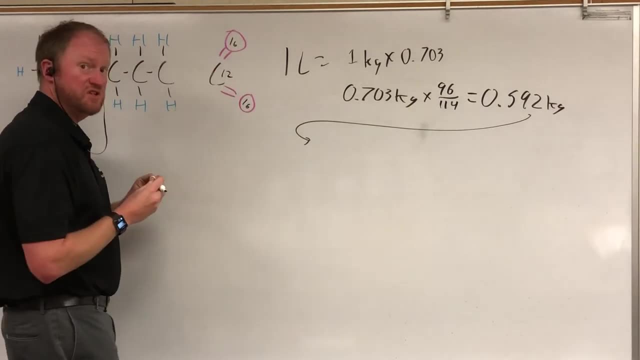 oxygen and the masses are are interesting here. so the carbon we said was 12, the oxygen has a mass of 16, so 16 and 16 is 32 plus the 12. so if we compare that so we have a total of 44 the carbon. 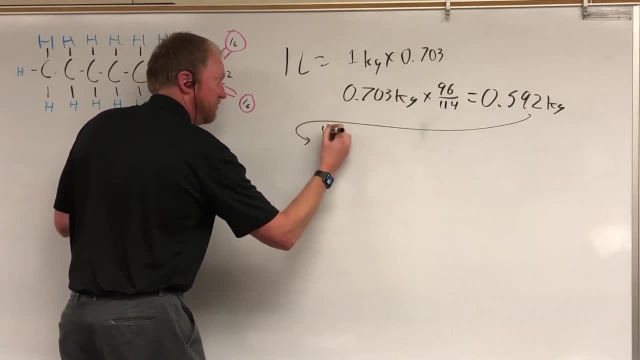 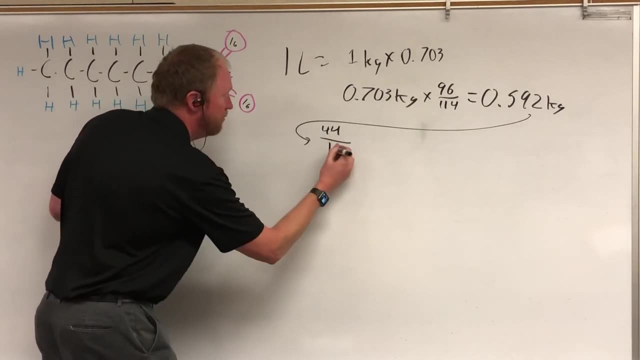 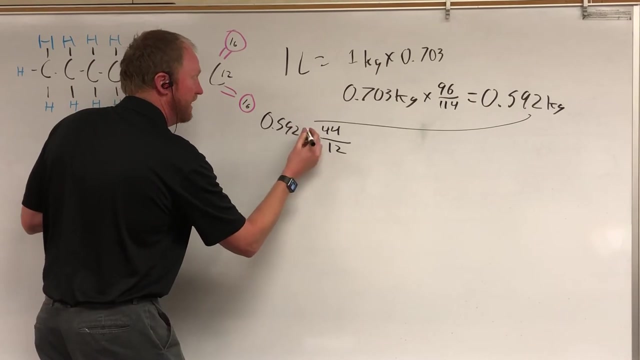 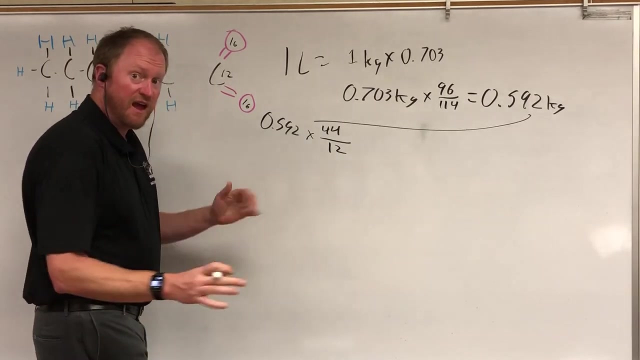 mass, the car of the carbon dioxide is 44 that you get out over 12. put in so we have zero point five. nine two kilograms that are carbon in the gasoline. you multiply that by 44 over 12 to find out how much carbon dioxide you're gonna get. 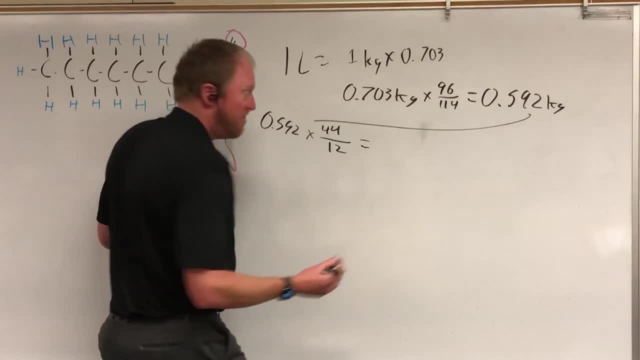 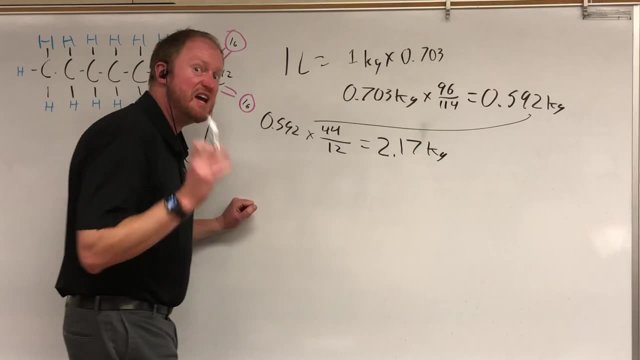 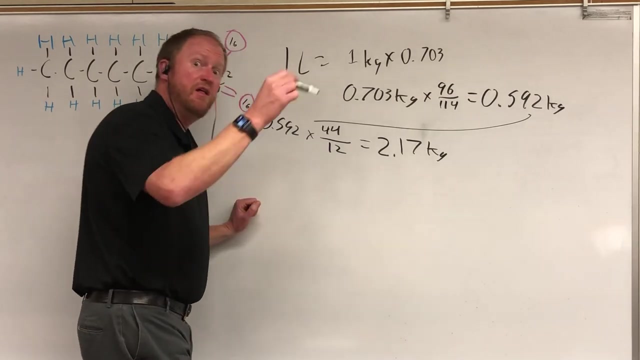 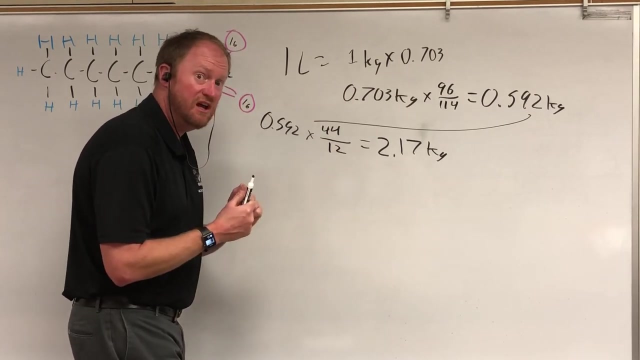 when you burn that and you find that you end up with two point one, seven kilograms of carbon dioxide. yes, the carbon dioxide coming out of the tailpipe of your car is heavier than the fuel you put in, and the reason why is because most of the weight is in the air. 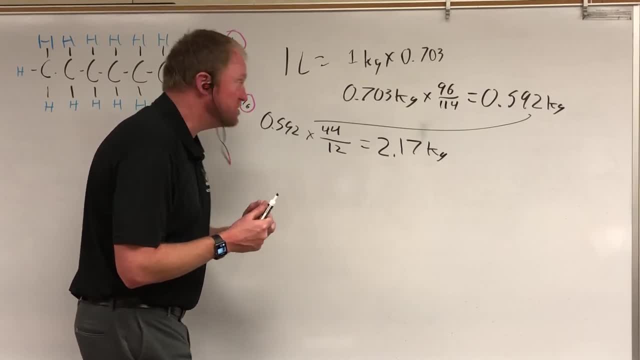 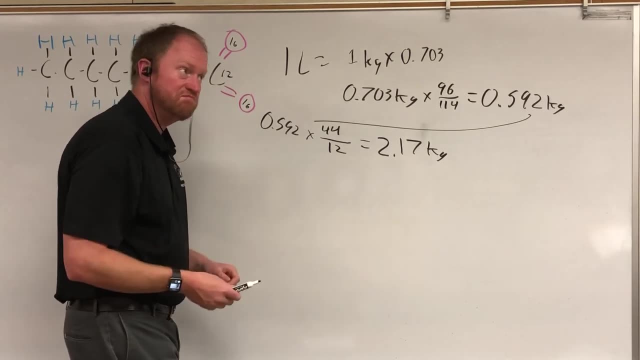 that is sucked into your engine, that oxygen is heavier than the fuel you put in. than the fuel, you don't notice that because the fuels a liquid and gas is a gas, but the carbon dioxide coming out of your engine is actually more than the weight of the fuel going in. makes you think: now, if you want to, so for every. 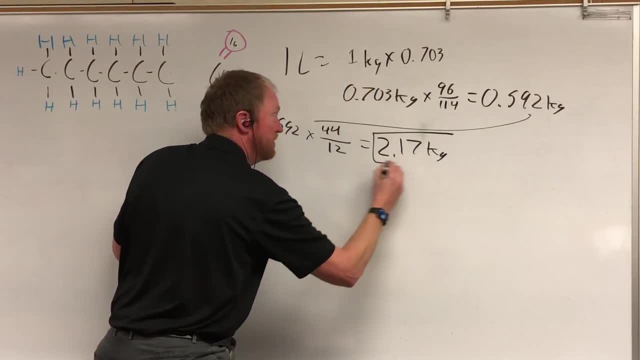 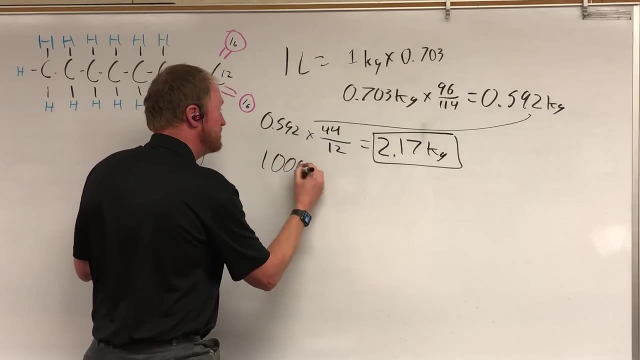 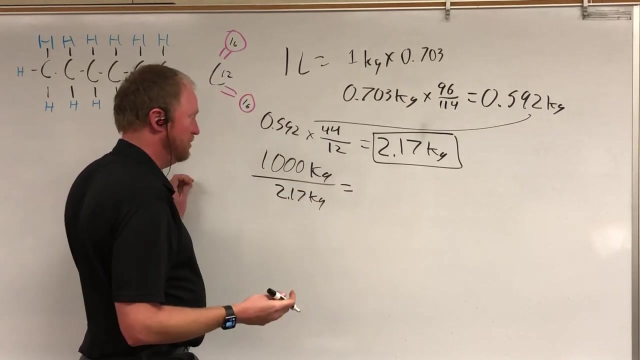 liter of gasoline that you burn, you produce two point one, seven kilograms of carbon dioxide. let's just take this a step further. so a metric ton is a thousand kilograms, and if you want to know how many liters it takes to get a thousand kilograms, well, you just divide that by two point one, seven kg, and you're gonna find that you